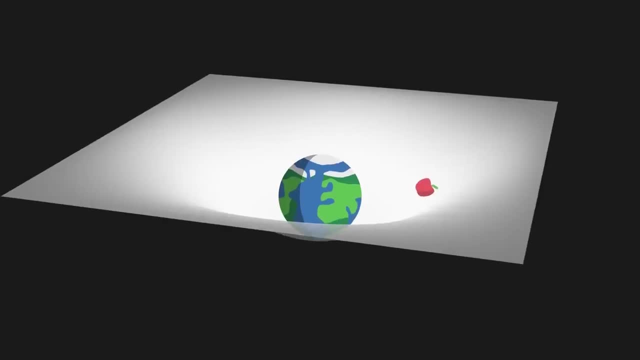 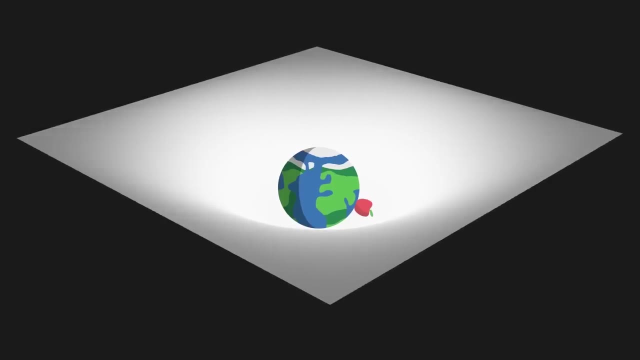 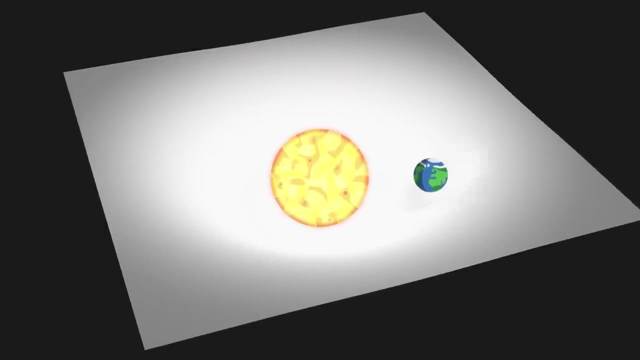 By deforming the fabric under their weight, the more massive objects pull everything in their direction, like marbles in a bowl. At first, this image seems to have two advantages: It is very simple and intuitive, and it helps us understand that bodies attract each other indirectly. 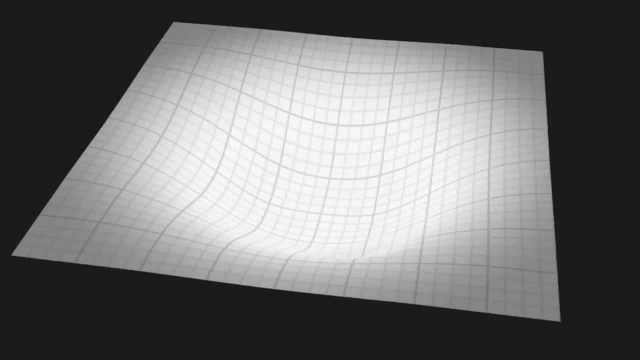 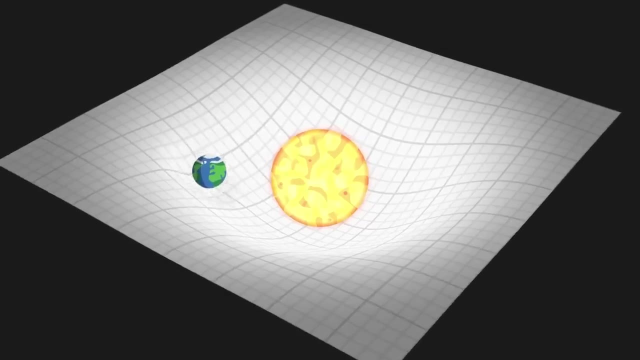 through an underlying fabric, spacetime whose geometry can be altered. However, although it is extremely widespread, However, although it is extremely widespread, However, although it is extremely widespread, this way of presenting general relativity has a large number of problems which make it not very rigorous. 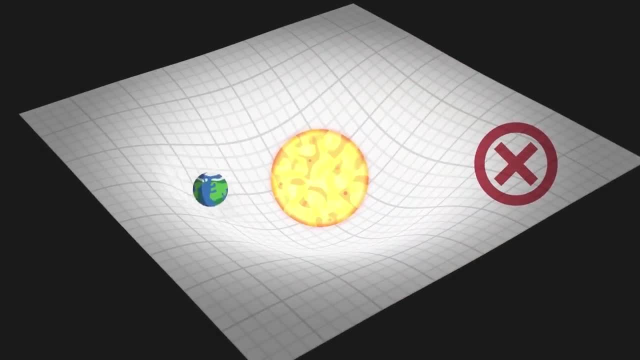 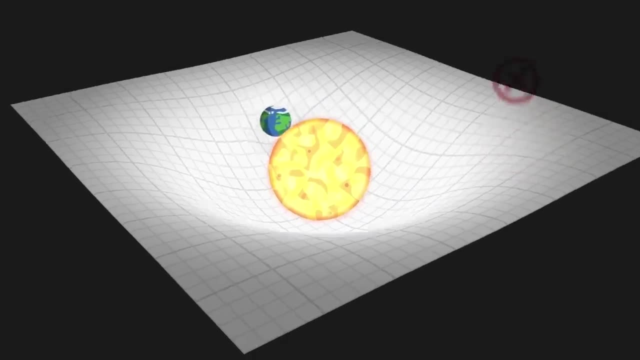 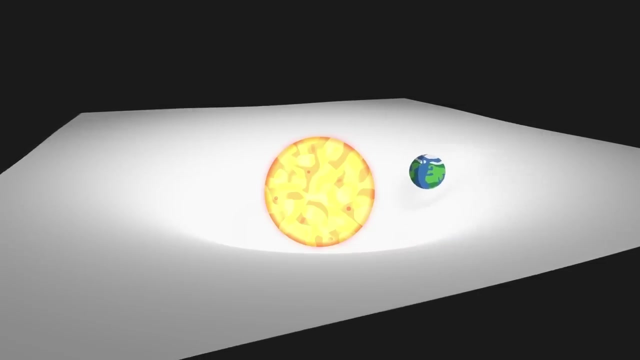 In this video, we will try to improve this image by making four major changes. To begin with, the image of the elastic sheet seems to indicate that objects are placed on spacetime like marbles, while in reality, spacetime is the fabric of the universe that contains them. 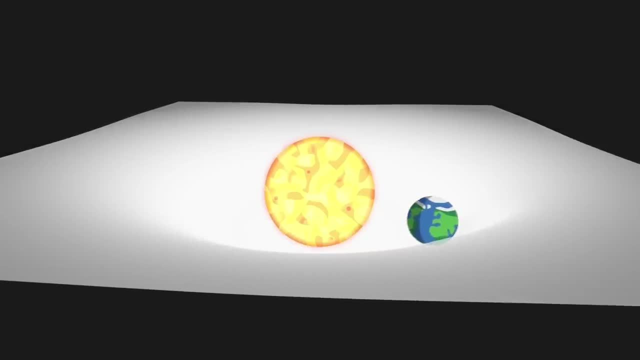 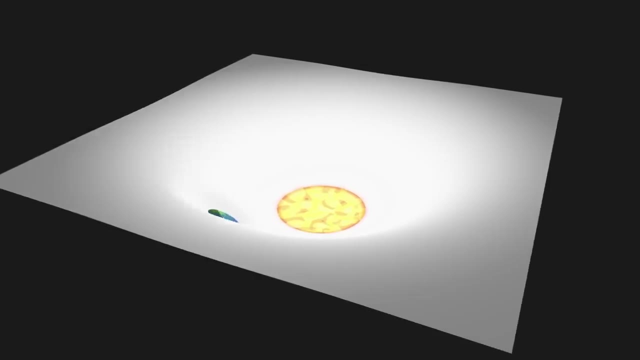 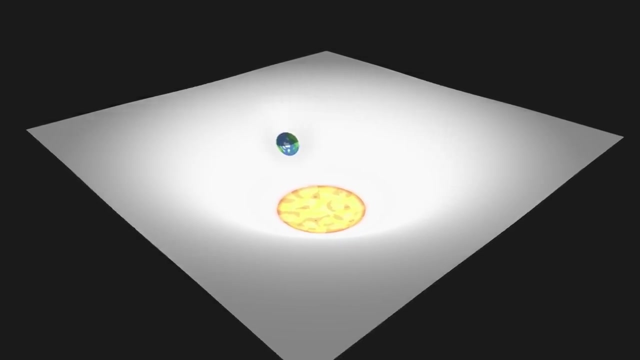 Therefore, one improvement that we can start with is to flatten objects onto the surface so that it is clear that they are not exterior but contained within spacetime. Next, one of the biggest problems with this representation is that it sort of explains gravity by gravity. 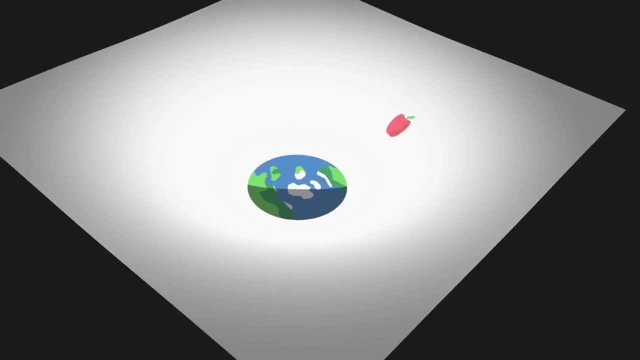 To the question why does the apple fall on earth, this visualization seems to answer that it is because the apple is flat. To the question why does the apple fall on earth, this visualization seems to answer that it is because the apple is flat. 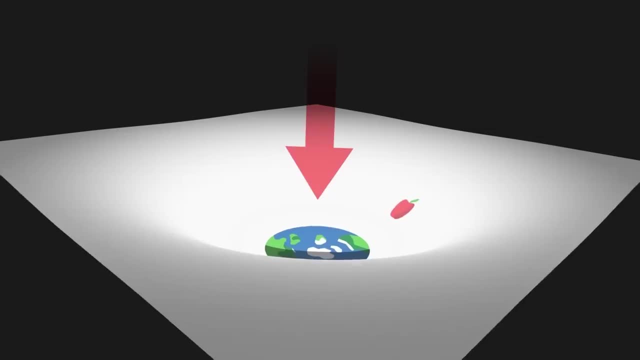 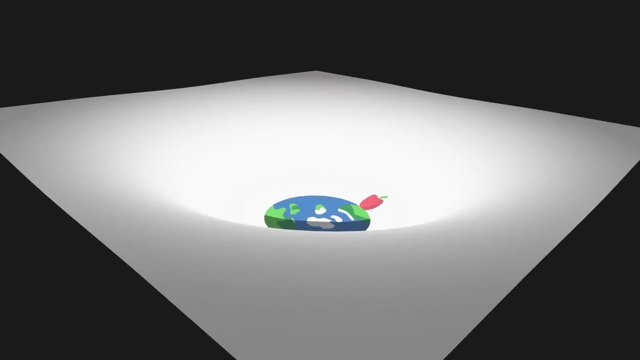 The apple is pulled downwards, which causes it to fall like a marble in a bowl. But it is not acceptable to explain gravity inside spacetime using gravity outside spacetime. We hence have to find a better explanation. In particular, it is more rigorous to say that if objects follow the well created by the earth, 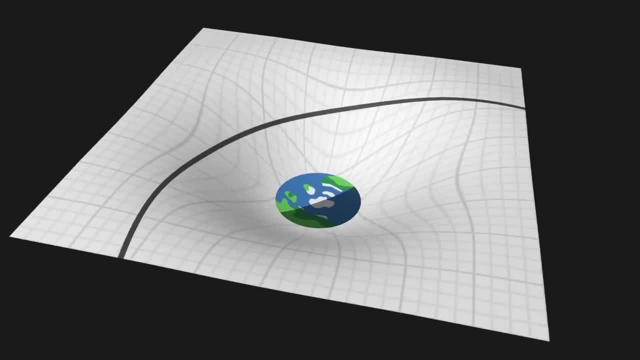 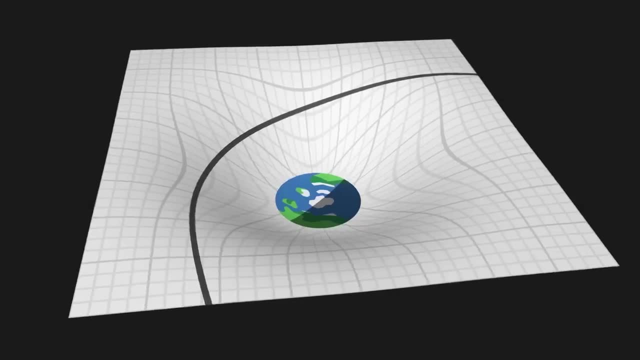 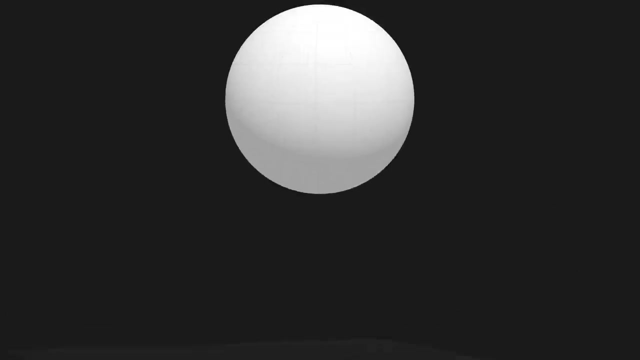 it is because they move in a straight line, but within a curved geometry. When they fall, objects move straight ahead, but the curvature of spacetime gives us the impression that these trajectories are deflected. To understand, we can imagine the surface of a sphere on which two ants would head north. 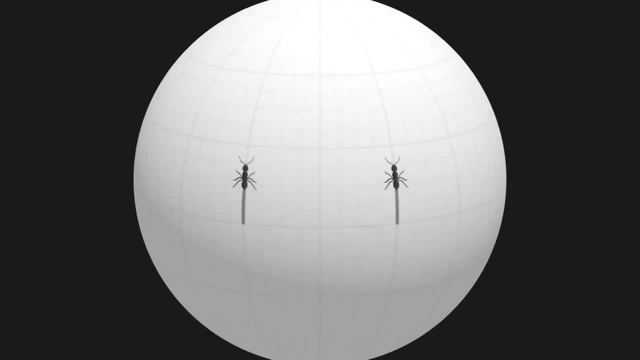 At the start, the two paths are parallel and we might think that, as they progress straight ahead, the two trajectories will never cross. However, the two ants end up meeting at the north pole. This is possible thanks to the curved geometry of the sphere. 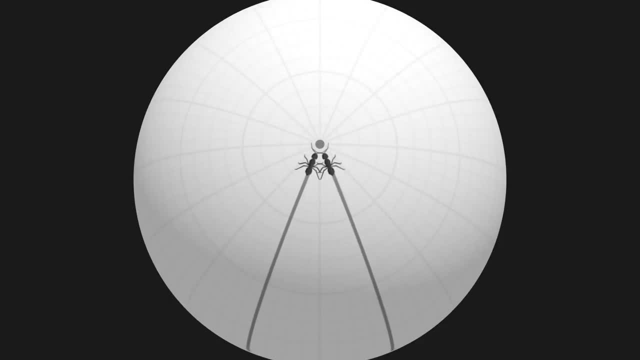 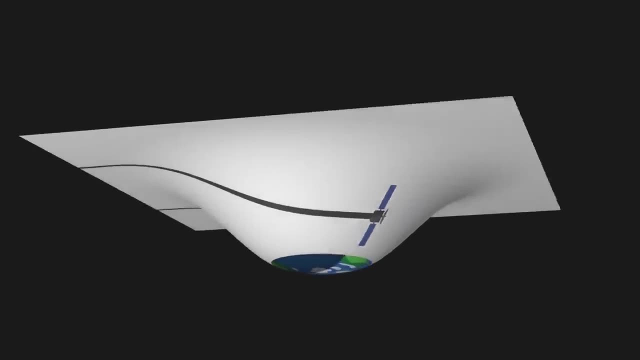 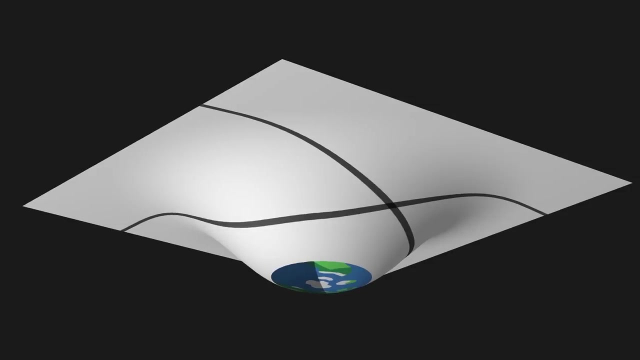 on which straight lines tend to get closer to one another. Inside spacetime, the phenomenon is similar and objects seem to attract each other when they are simply following the curved geometry in straight lines. However, this picture of an elastic sheet is still misleading. 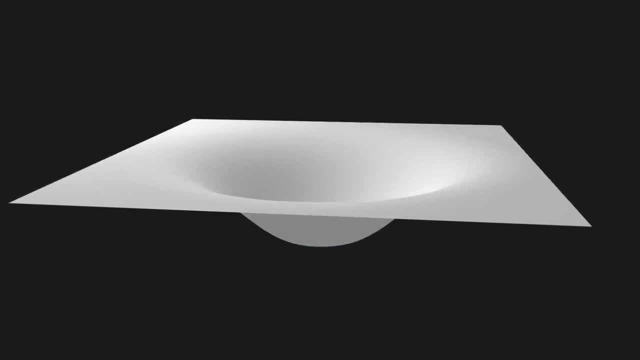 Indeed, one could think that if spacetime can bend, it is due to the existence of a higher dimension. Here, for example, the two-dimensional sheet seems to bend into a third dimension. In reality, this is not the case, and the mathematics of relativity do not require any higher dimension for the universe to bend. 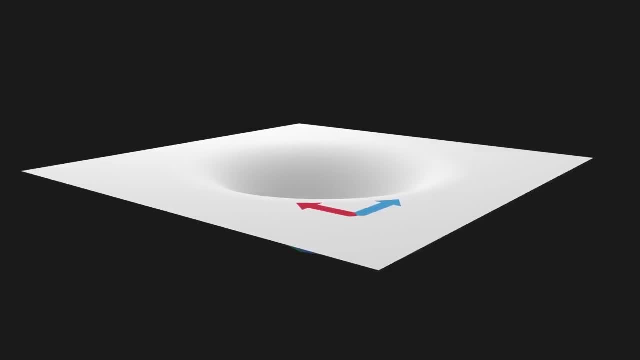 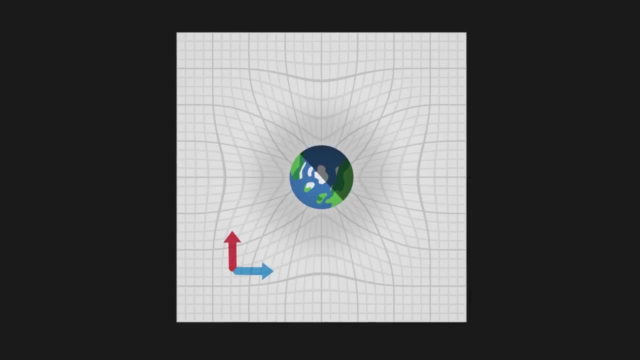 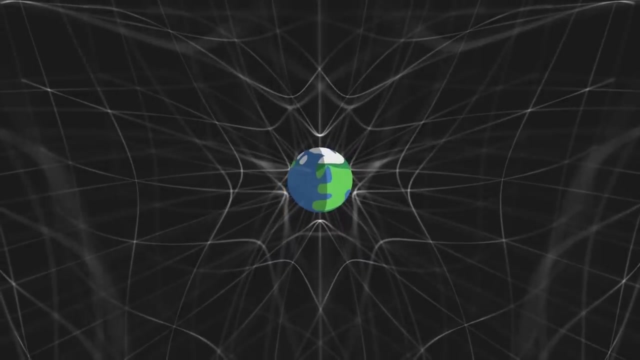 It is therefore preferable not to represent this sheet seen from the side, but rather from the top, with a grid to illustrate the curvature. While we are here, this also allows us to restore the three dimensions of space in which we live. Finally, the most important issue with this representation: 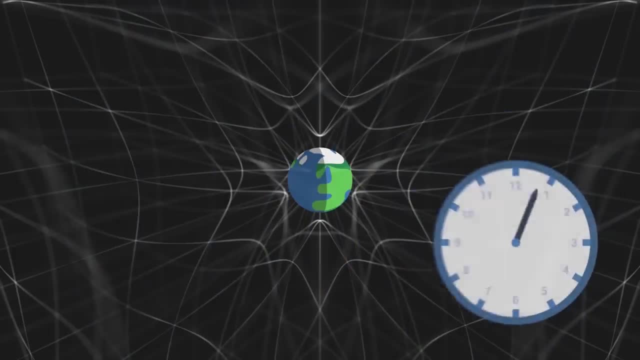 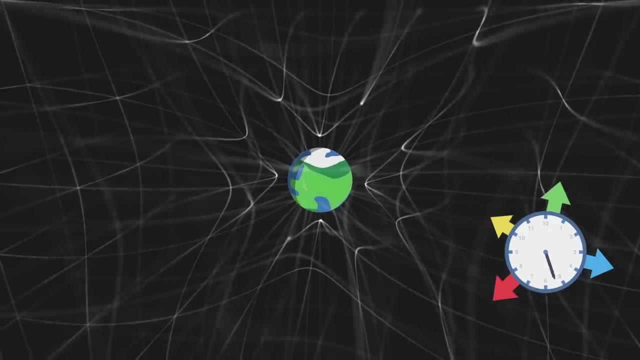 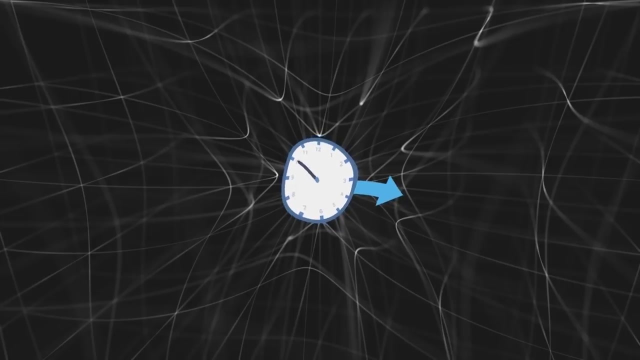 is the fact that our diagram completely ignores the time dimension. Spacetime is an object with four dimensions: three dimensions of space, but also one dimension of time which can equally bend and curve. Faithfully rendering a four-dimensional geometry is strictly impossible. 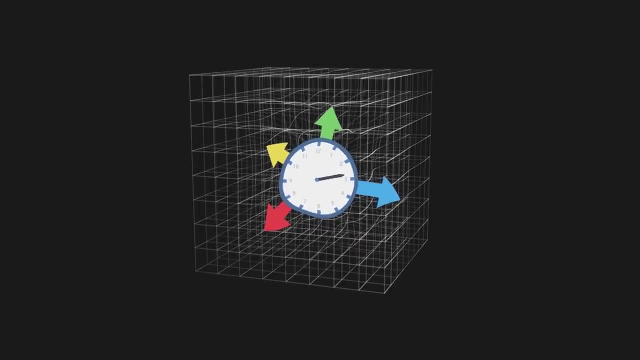 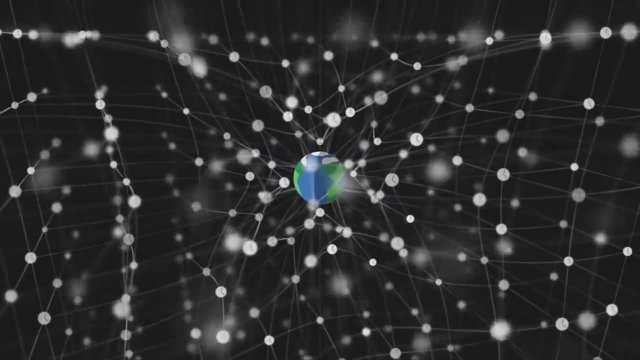 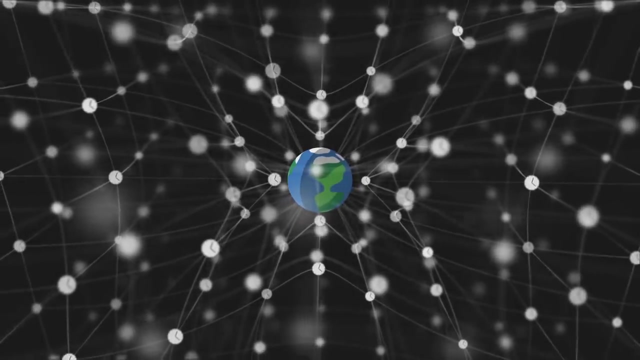 and we therefore have to find a trick. A first idea would be to add small clocks to our diagram at each point of the grid. In this way, the space grid becomes a spacetime grid, and we understand that time can flow differently depending on where we are. 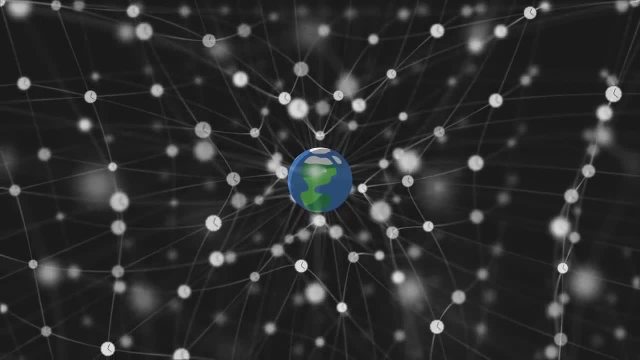 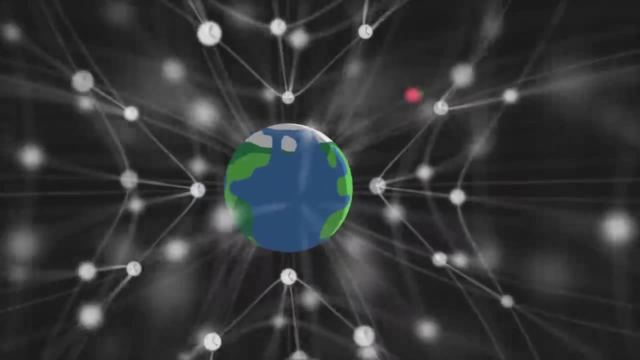 That being said, adding clocks to our diagram doesn't give us much more intuition and, in particular, we still don't really understand what causes objects to fall. If we drop an apple, for example, why does it start to move towards the Earth? 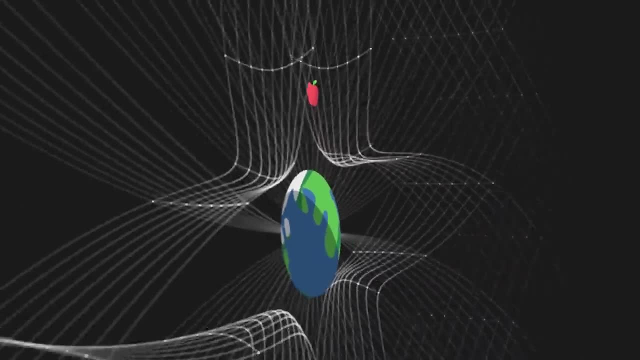 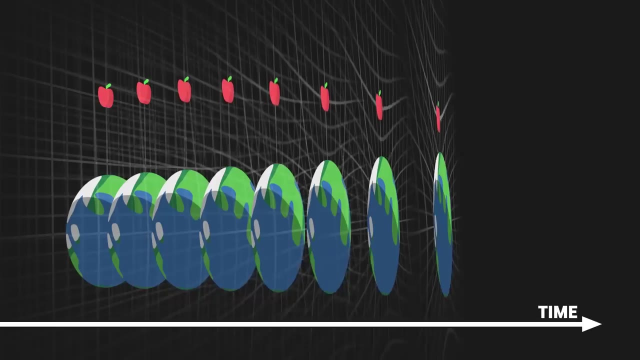 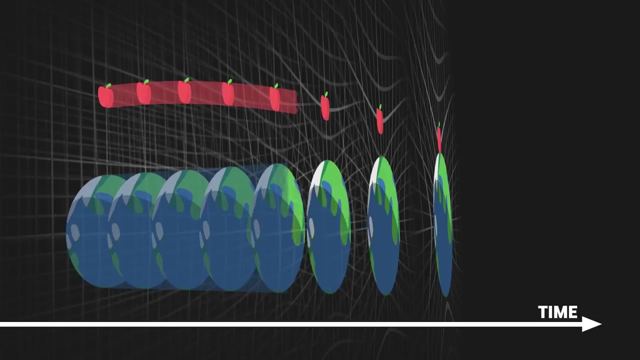 To really understand, it is necessary to remove one dimension of space to represent the dimension of time. In fact, it is the time component of the curvature Which explains gravity. With such a diagram, we see that the apple is always in motion. 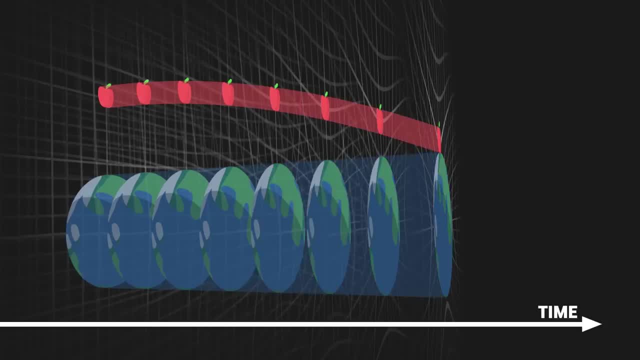 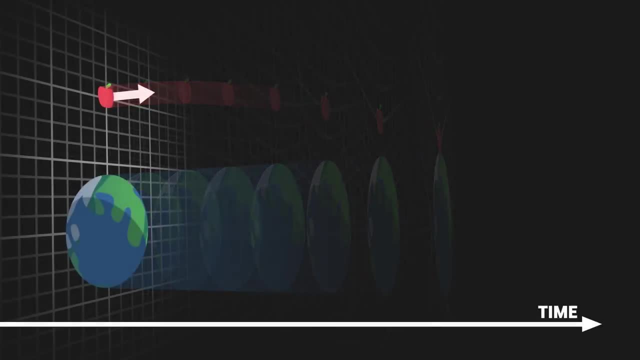 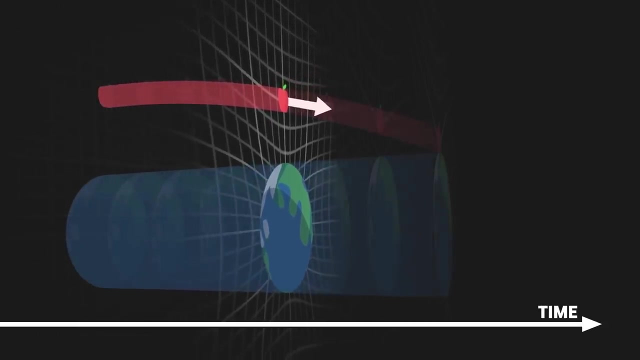 Even when it has no speed at the start of its fall, the apple is still moving in time. It progresses towards the future. When no force is applied to the apple, the curvature of spacetime will gradually bend its trajectory between a temporal speed towards the future. 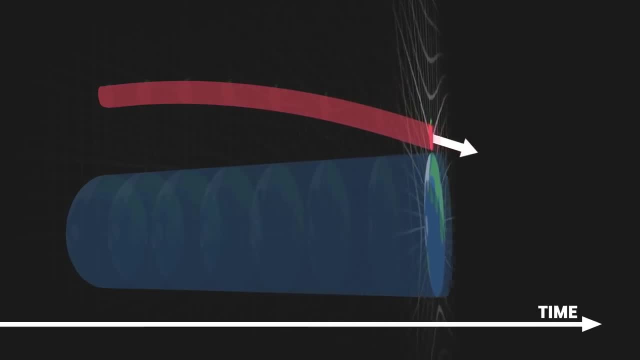 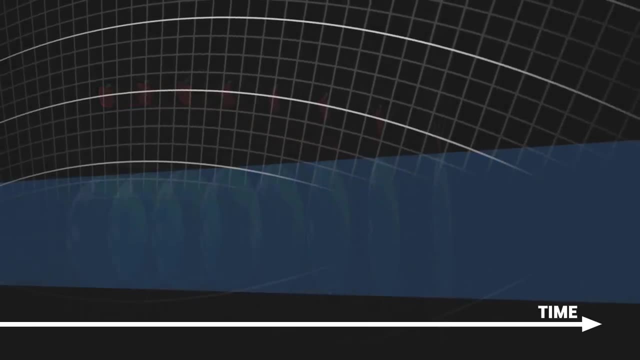 and a spatial speed towards the ground. The apple moves in a straight line, but the curvature of spacetime rotates the orientation of this straight line between time and space. We therefore understand that if the apple falls towards the ground, it is because it started with a speed through time. 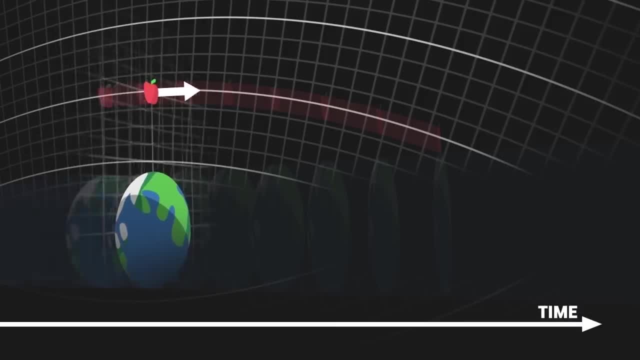 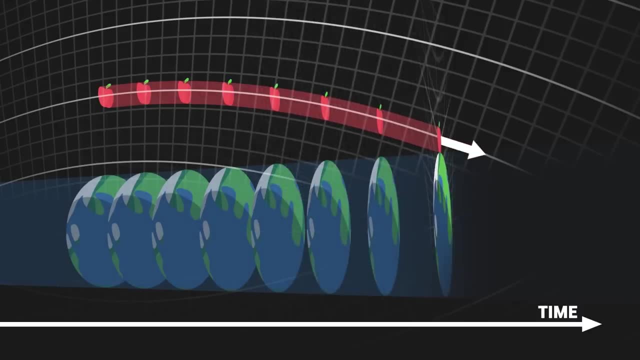 The curvature of spacetime generated by the Earth converts this temporal speed into a spatial speed. Having said that, as human beings we do not perceive the temporal speed of objects. When an apple is dropped, it appears to us to be motionless. 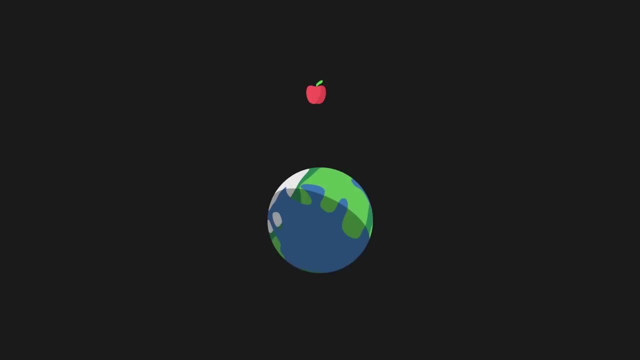 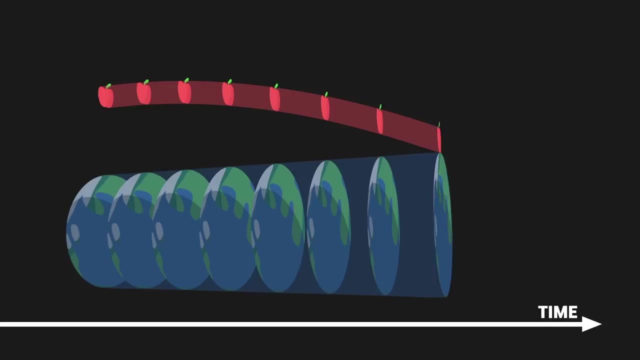 We do not perceive the fact that it has a motion through time. From our point of view, we experience the world instant after instant, And this diagram where objects form tubes over time, world lines, is not very intuitive. Our last step will therefore be to slice this diagram. 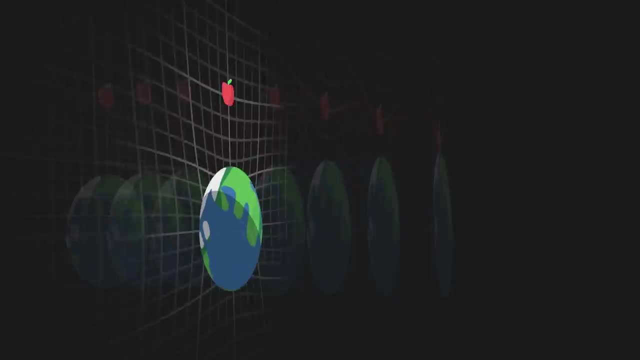 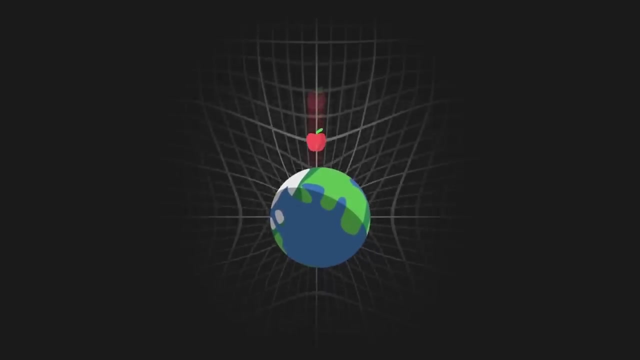 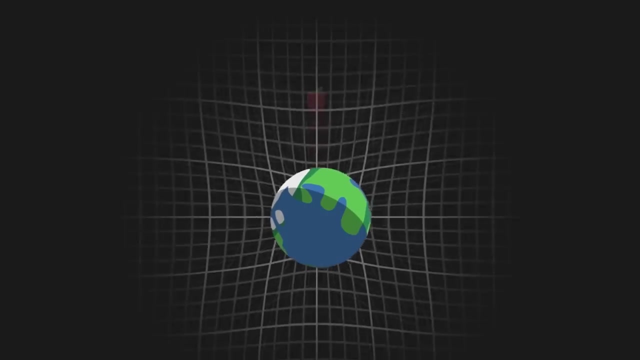 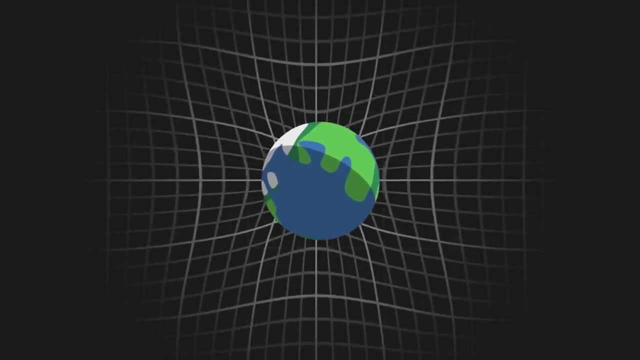 to cut it up instant by instant in order to form an animation which includes time. The curvature of the universe, which causes straight lines to dive into the universe, becomes a movement of contraction. The rate of this contraction is constant and perpetual because the curvature of spacetime 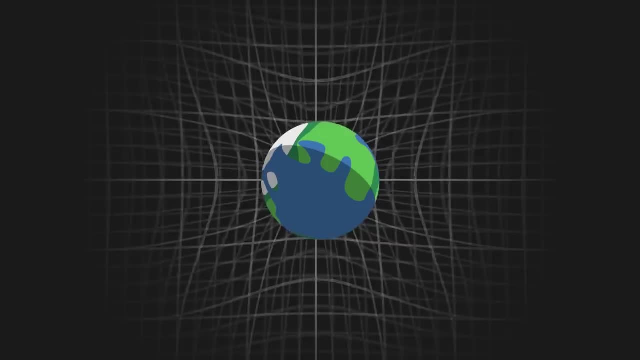 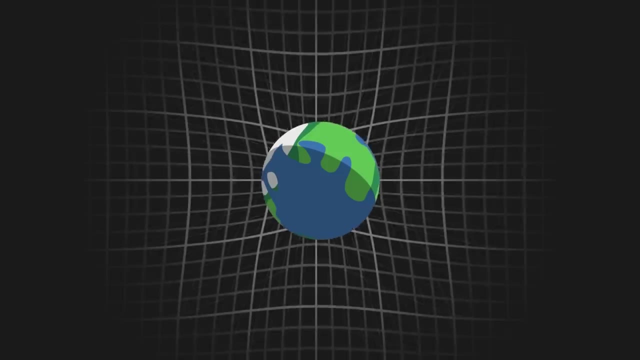 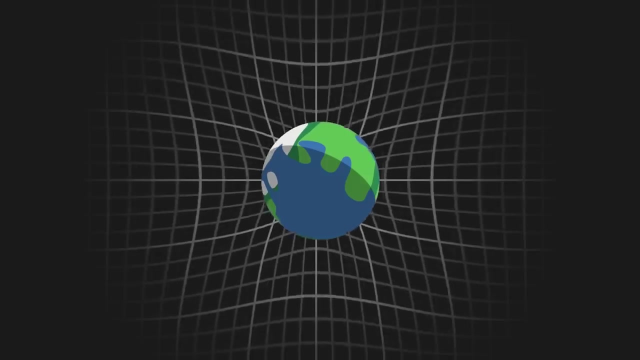 which depends only on the mass of the Earth, is always the same. However, it is very important to understand that the geometry does not really contract. It is the fact that straight lines get closer together that gives this impression of contraction. The phenomenon is quite similar on the surface of a sphere. 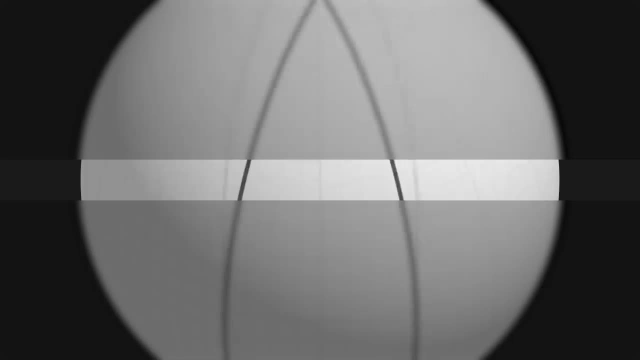 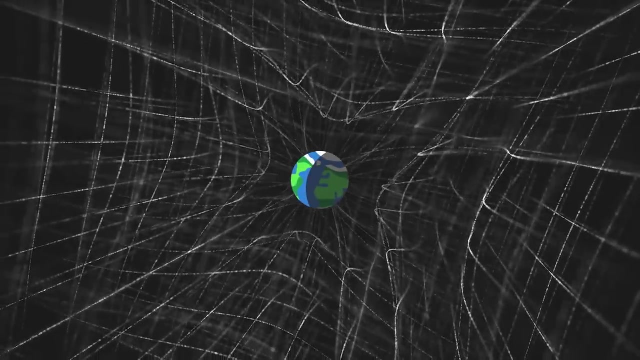 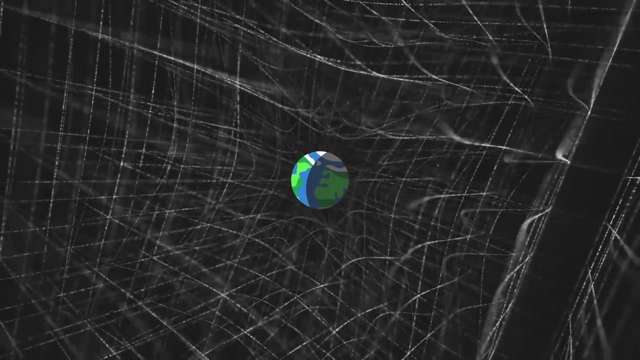 The curvature is constant on the sphere, but the straight lines seem to be perpetually getting closer together. It is this representation which I find to be the most appealing for visualising general relativity: The Earth, because it is very massive, deformed spacetime. 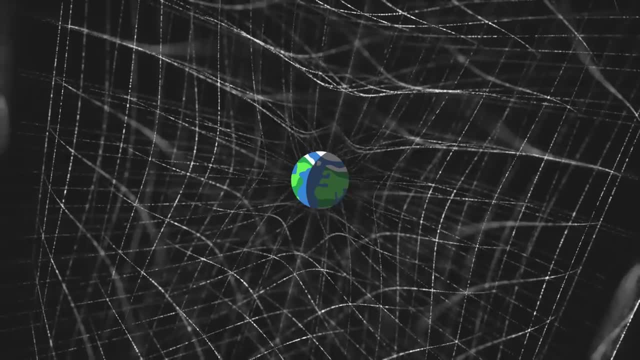 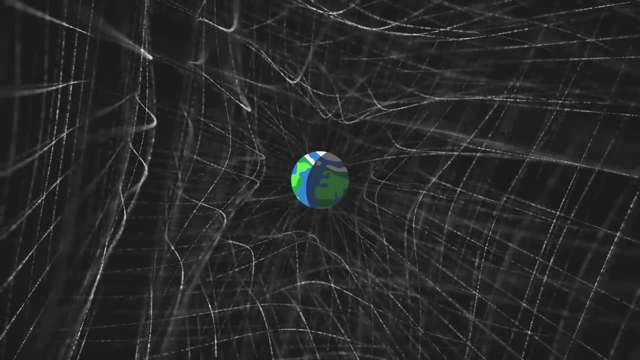 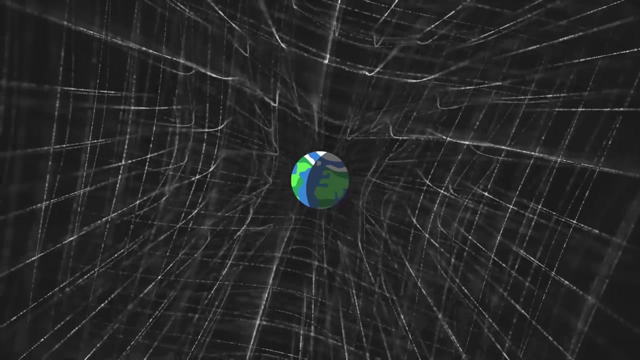 giving it a curvature. For us, the curvature of spacetime appears as an endless contraction of the grid. In technical terms, we say that the volume contained between geodesics shrinks over time because of the curvature. This grid that shrinks represents what we call inertial frames. 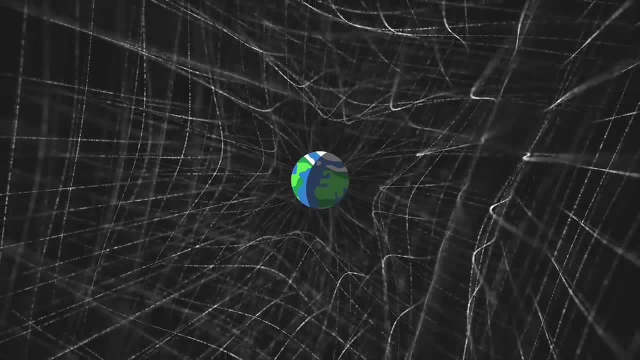 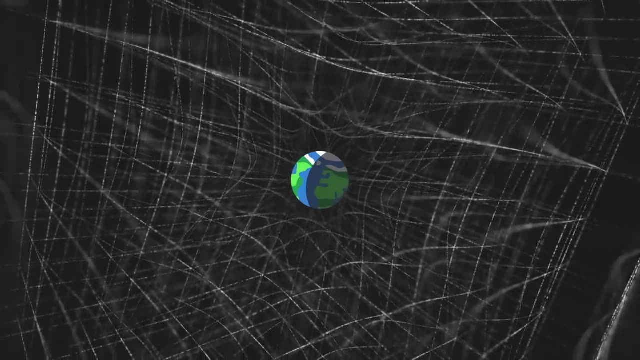 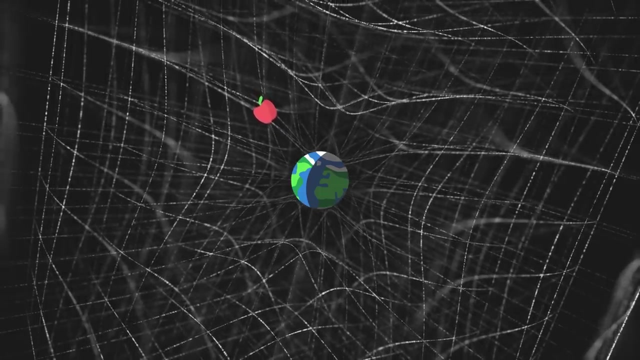 frames in free fall With respect to this grid. a body that is not subject to any force will conserve its movement. Thus, if we drop the apple with no initial velocity, as no force acts upon it, it will remain motionless relative to the grid. 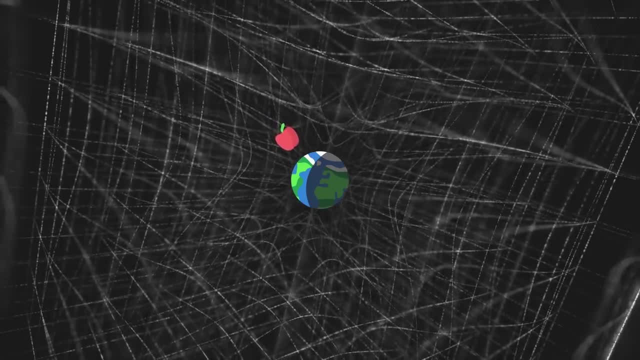 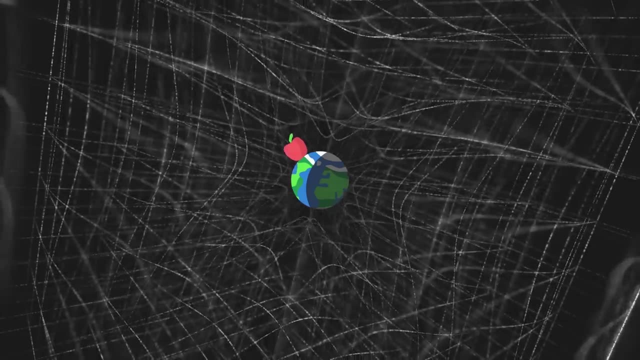 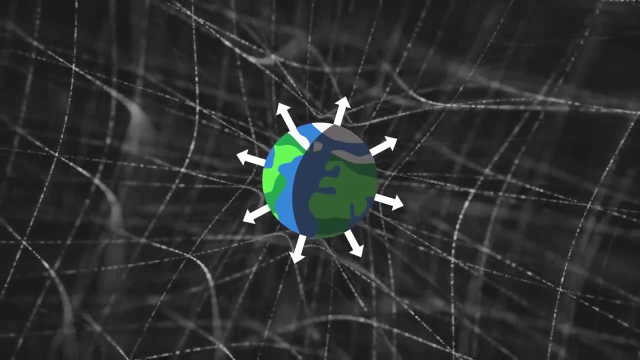 but as the grid contracts, the apple will fall. With this image of relativity, it is also easy to see that the surface of the planet is constantly accelerating upwards, because it is always going against the natural movement of the grid. Finally, if we throw an object sideways, 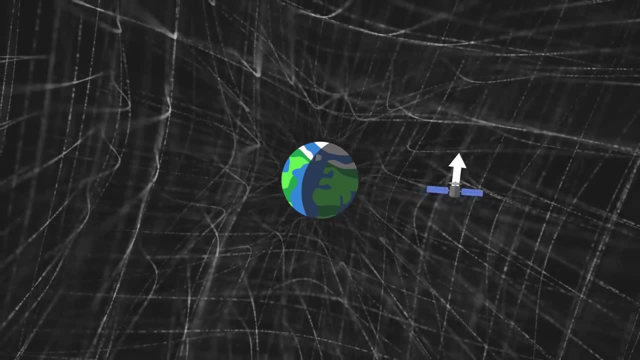 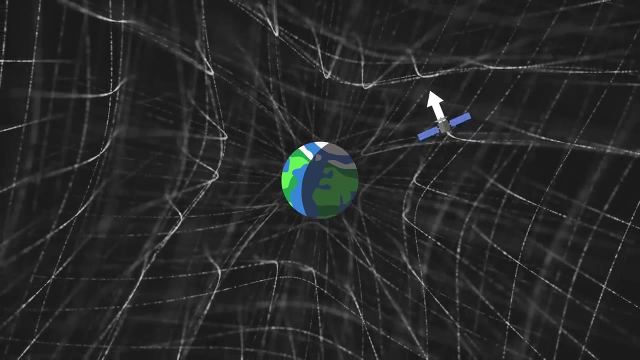 with an initial velocity. no force is applied on it and it will therefore continue in a straight line within the grid. But as the grid contracts, the object is constantly pulled back towards the Earth. That's exactly how the Moon orbits the Earth. 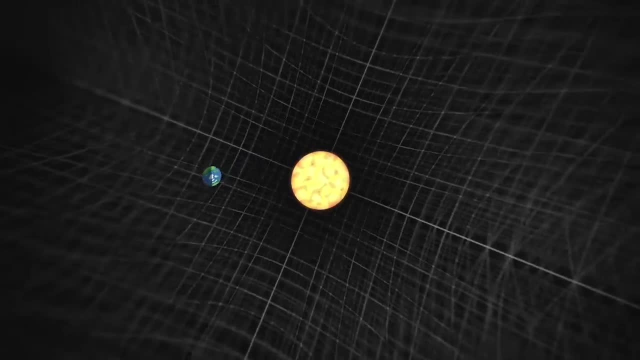 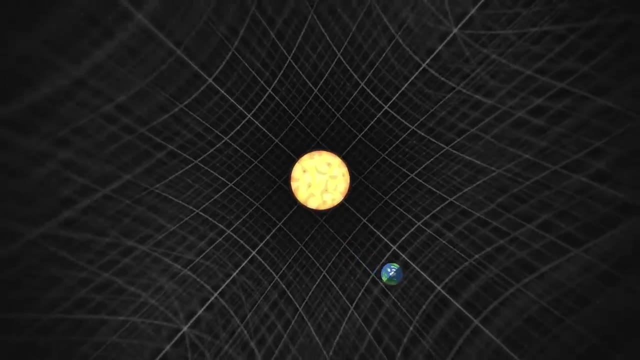 and the Earth orbits the Sun. NASA Jet Propulsion Laboratory- California Institute of Technology.